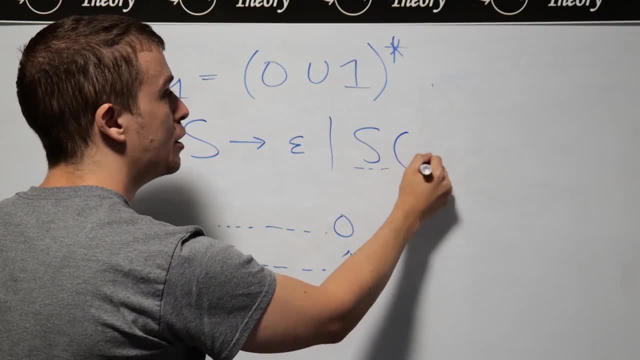 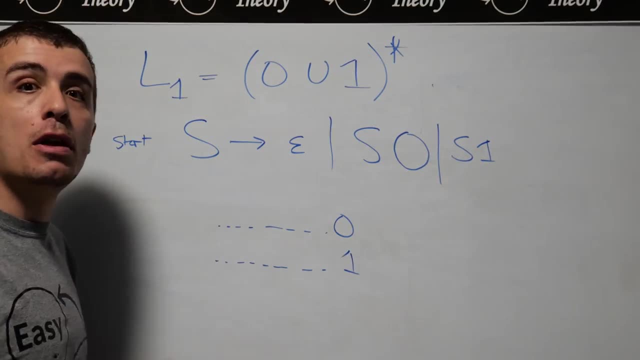 corresponding to this s right. here. we need to allow ourselves to make a zero afterward, but also allow ourselves to make a one afterward, And so, therefore, this is a context-free grammar for this particular language. Now, there are many other types of context-free grammar, but this is a context-free grammar for this particular language. Now there are. 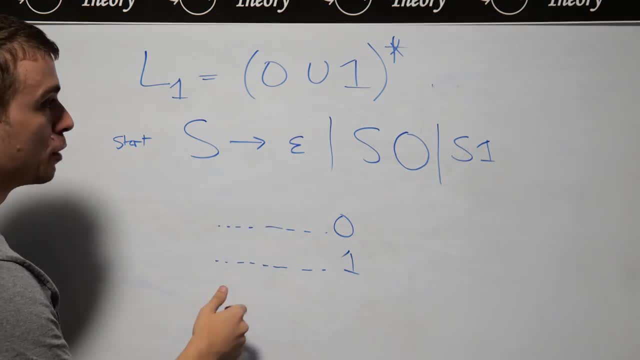 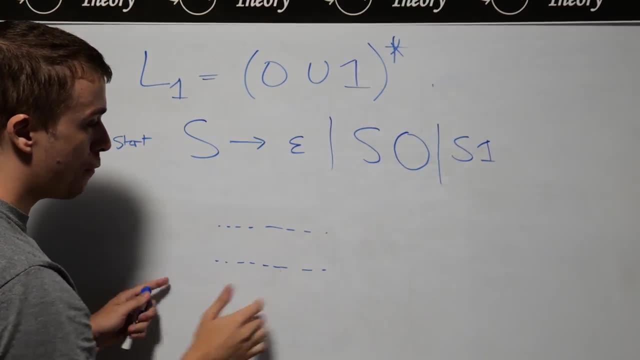 many other types of context-free grammars we could have made. We could have had some other variables right here. we didn't have to put the zero on the end, we could have put it on the front, because the same logic will apply. if we have made some strings so far, We can always stick a zero or a one on the. 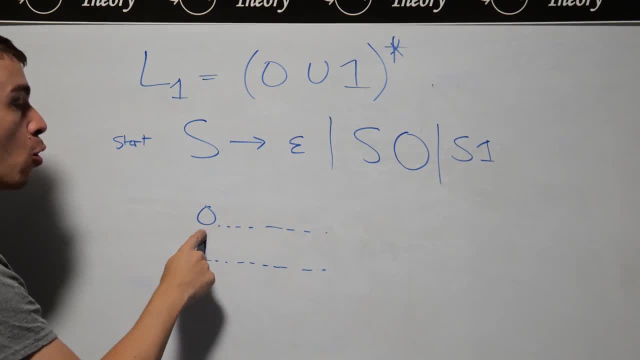 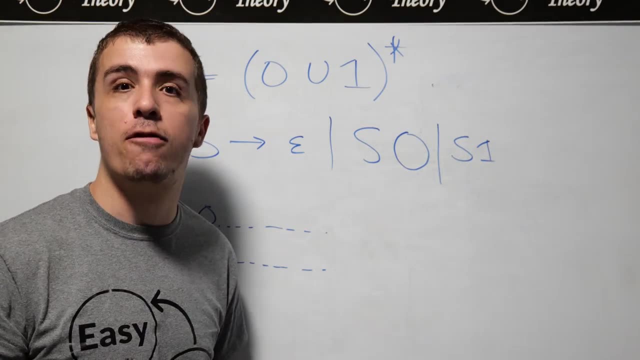 front and every string is either the empty string, or it starts with a zero, or it starts with a one. So there are many different context-free grammars that we can make, but this is one of them for L1.. Okay, let's make a context-free grammar for this language. 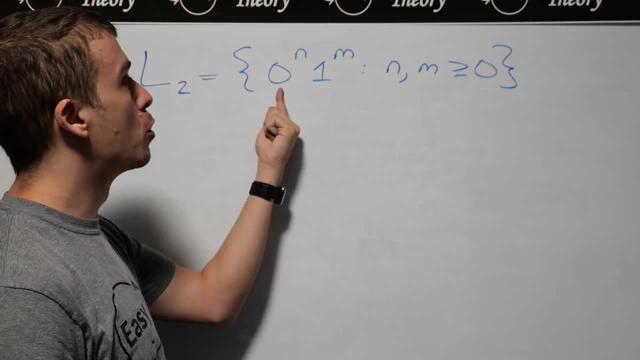 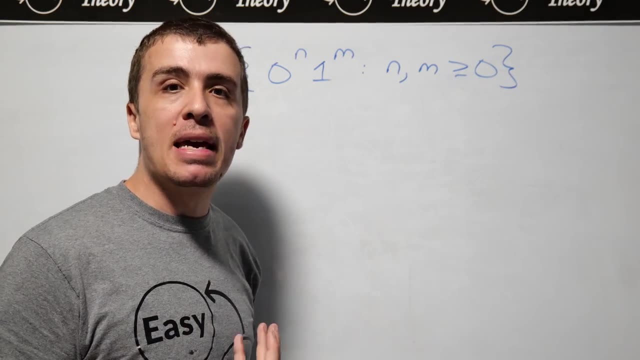 L2, which is the set of strings of the form 0 to the n, 1 to the m, where n and m are at least zero. So one thing that you should be aware of when making a context-free grammar for a language. 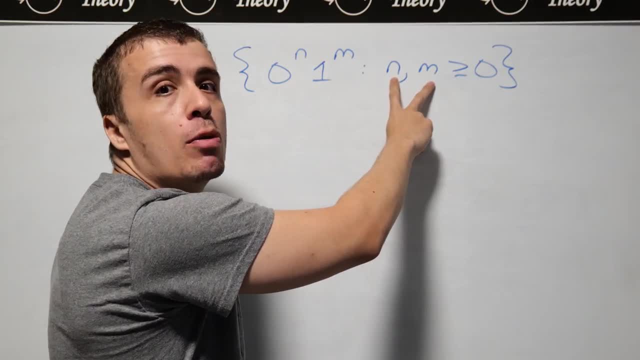 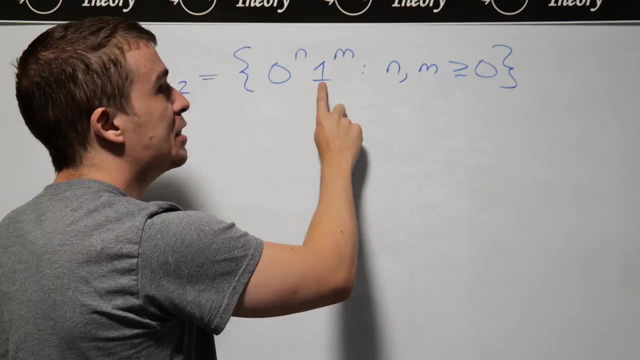 that's given to you is: what are the relationships between the counts here? So the count n here is relating the number of zeros. well, it is the number of zeros and m is the number of ones here, And note that there's no correspondence between the n and m parameters. they don't have to be the same. 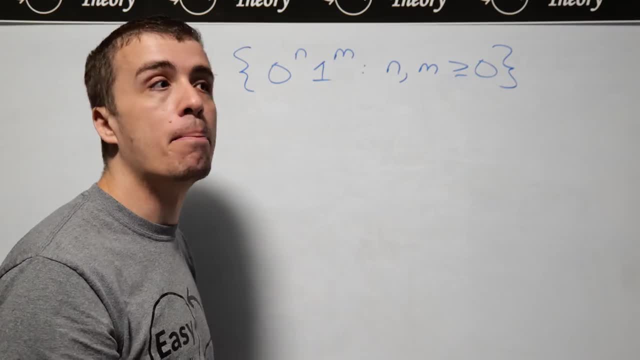 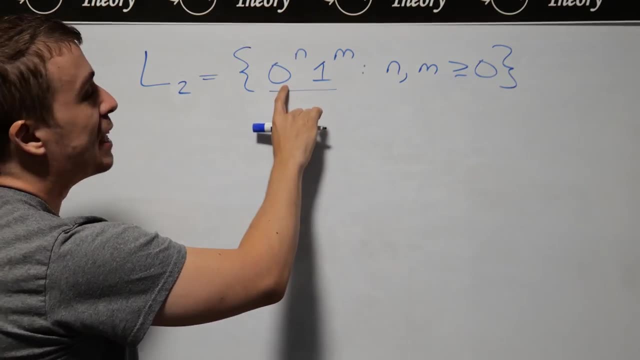 or different or anything. They're just independent numbers, And so therefore we can treat them completely separately. So every string in this language always has some number of zeros at the start and then some number of ones at the end, And so therefore we can actually write a regular. 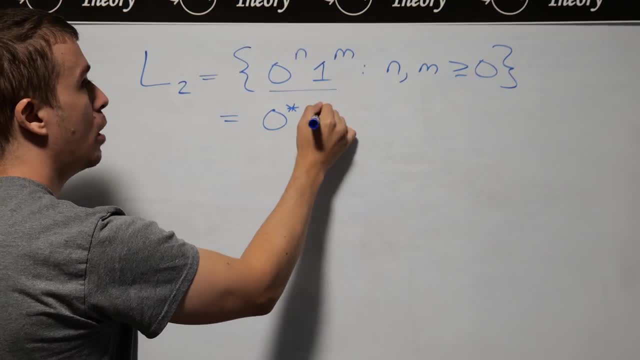 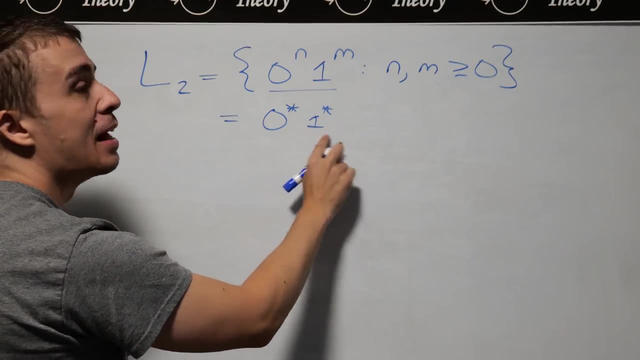 expression for this. We can just say that it's zero star. one star because it's just some number of zeros, any number that we want, because there's no restriction there other than being at least zero- and then followed by some number of ones, So we can make a context-free grammar for this. 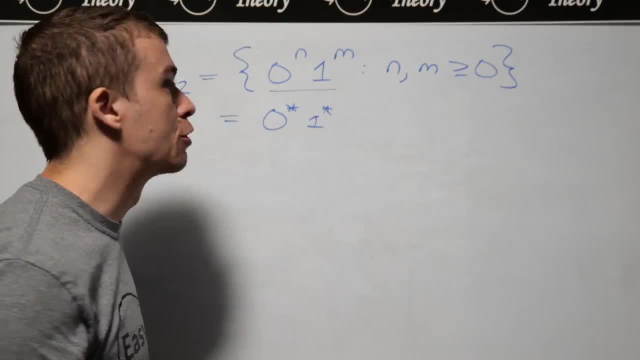 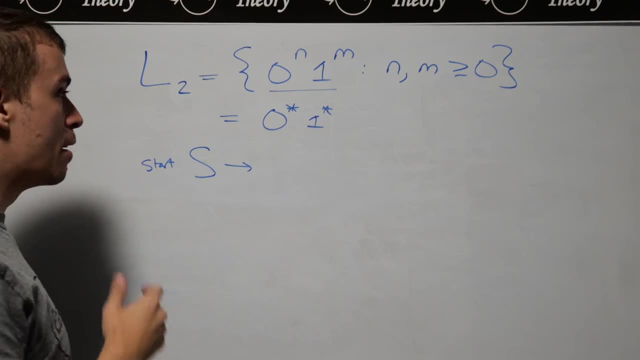 We can make a regex for this, But what we're after is a context-free grammar, So every context-free grammar needs a start variable. so let's make a start variable right here, And then what we want is that we need to generate some number of zeros and then, once we're done generating the zeros, 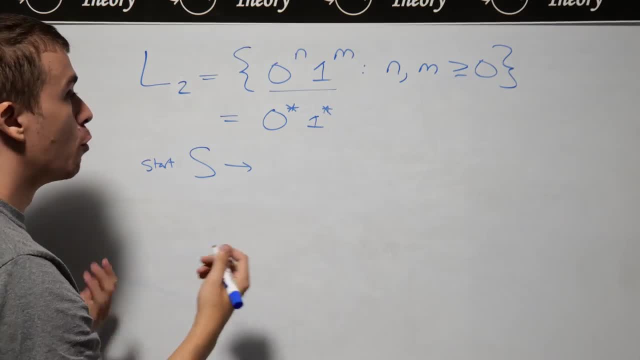 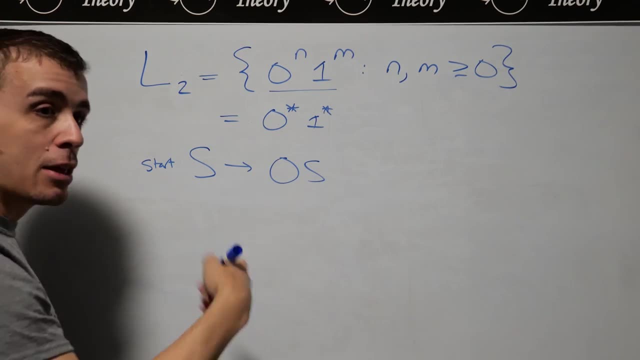 whatever that means, we need to be able to generate some more ones. So one thing that we can do is let's just make a bunch of zeros right here, by having a zero followed by s, which says you can add zeros on the front as needed. 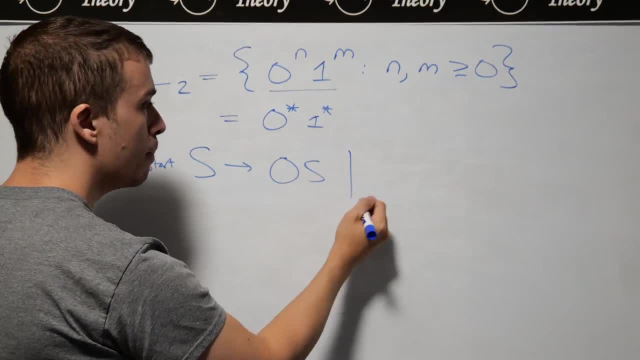 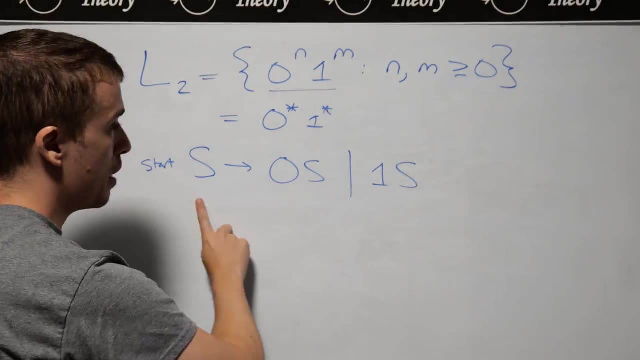 And then at some point later, we need to switch over to ones. But it'd be an incorrect idea to do this, because if we have this right here, where s is the start variable again, what can happen is that we can interchange these two rules, So therefore we could apply this rule, then this: 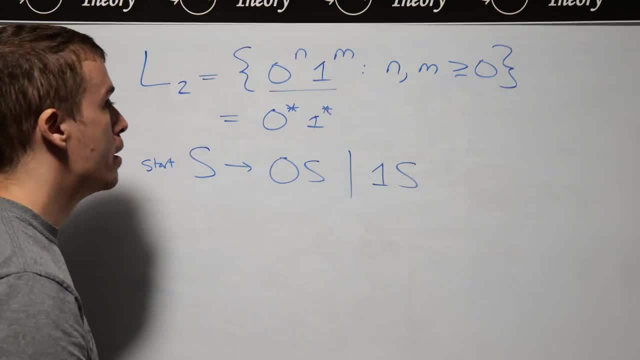 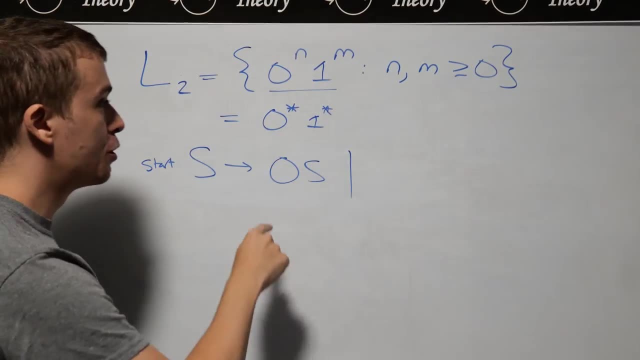 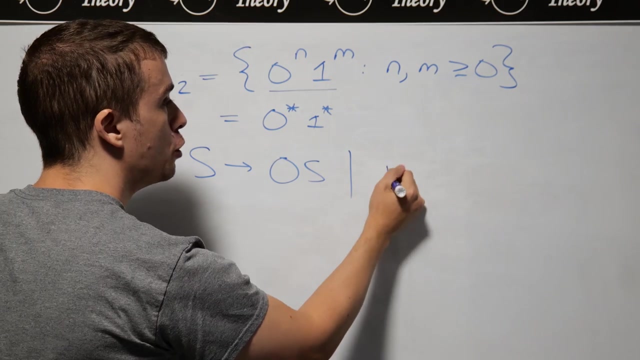 rule, then this one, and then just go back and forth as any way that we want, And this is a bad idea. So what we want to do is to go to some other place where we can't access this rule anymore, and then generate the ones there, And so what I'm going to do is I'm going to go to a 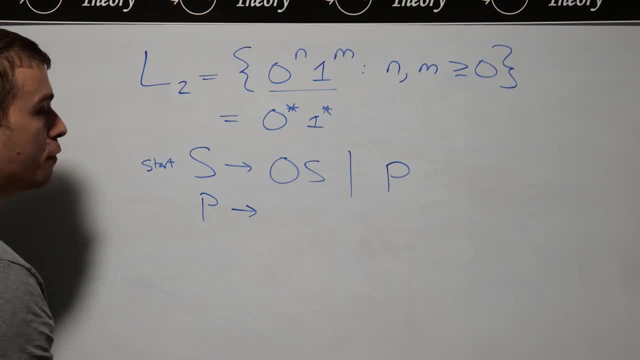 variable called p. So p is a completely new variable where I can now make the ones here. So, just like with the s variable, where it can make zeros, I can make ones here and there's no relationship other than the ones being after the zeros. And now, once I'm done, 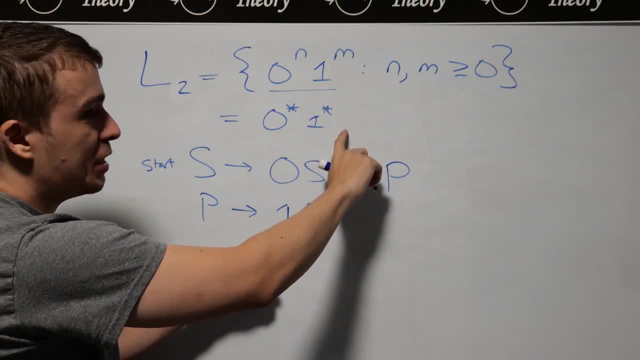 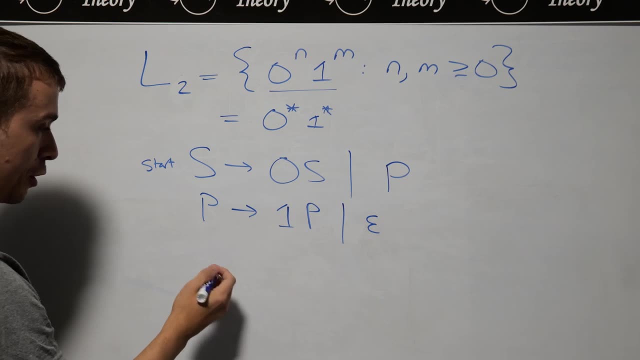 generating the ones. well, there's nothing after the set of ones here, and I can do this as a as many times as I like, So I need to be able to stop by making the variable go away. And so if we look at a particular example, so let's consider the string, say two zeros and a single one. 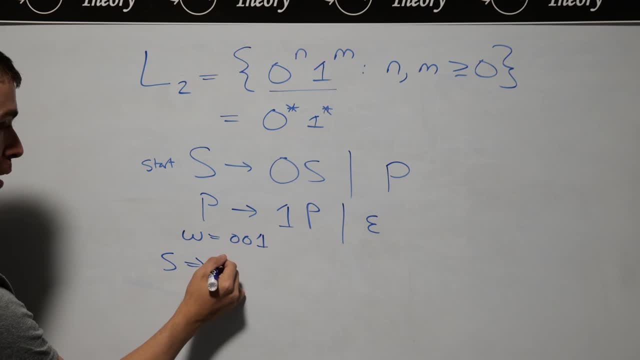 then a derivation will be: s goes to 0s. So I replace this s with 0s, which is this rule. Then I'm going to replace this s with another application of the same rule, So I get 0,, 0, s. 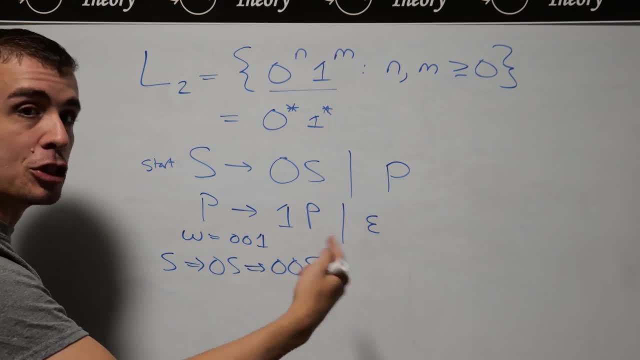 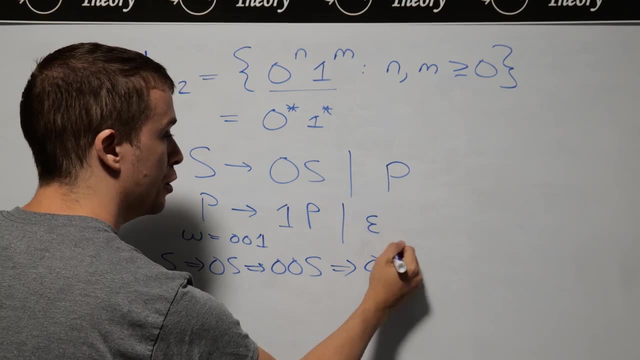 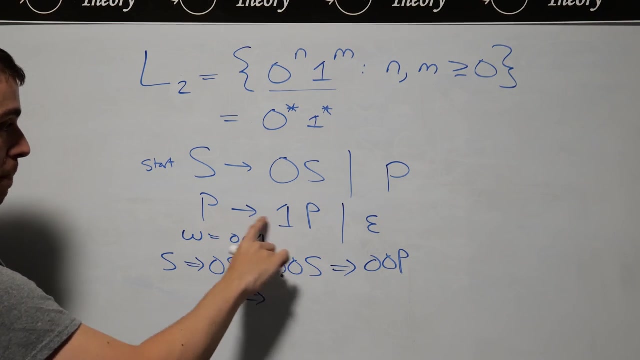 Then, now I'm done generating the zeros, I need to switch over to the ones, So I'm going to now replace this s with p, So applying this rule this time. So 0, 0, p looks like object-oriented programming. Then now I need to generate a one which is applying this rule. p goes to 1p, So 0,. 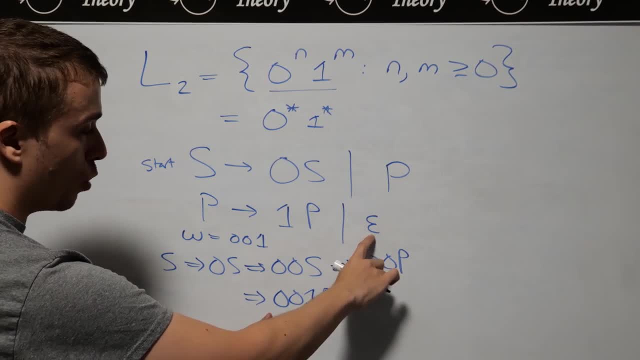 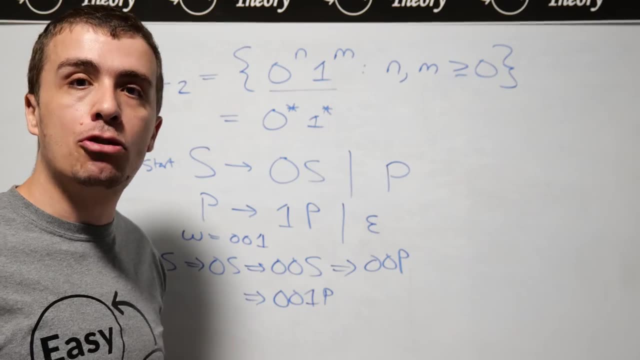 0, 1p. And then now I need this rule here, because every rule in the grammar otherwise always has a variable attached to it And we need to make sure that we have a variable attached to it. We need to make a string with no variables at all, only terminals, because that's what the 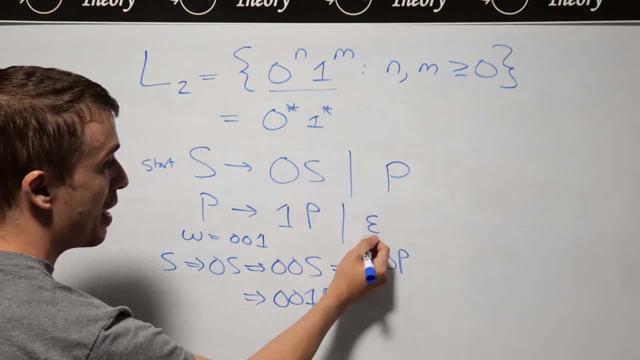 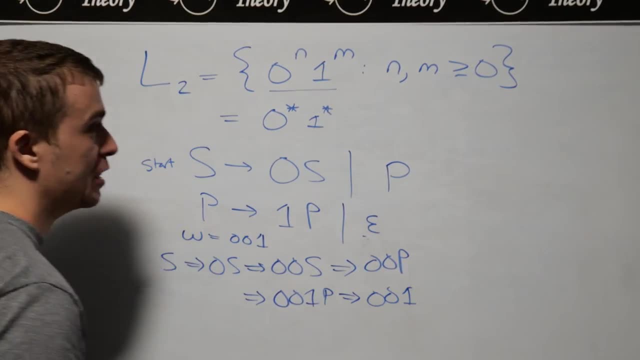 language of a context-free grammar is, And so now I'm going to apply this rule right here by making p go away, In other words, changing it to be the empty string, which is exactly what this is. And so, therefore, this is a context-free grammar for this language, which is the regex corresponding. 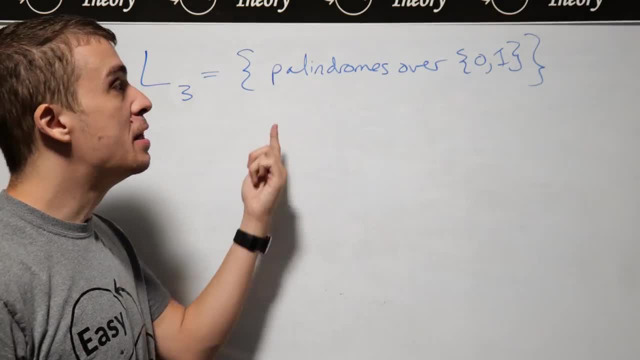 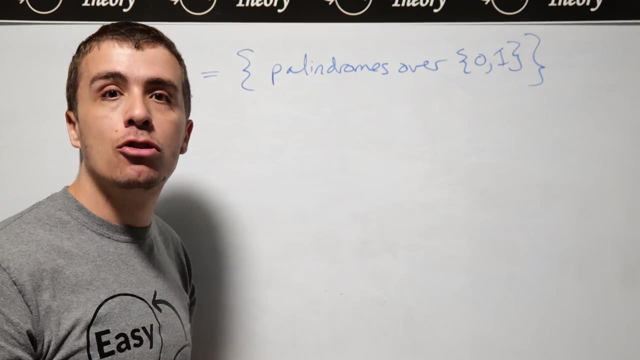 to 0 star. 1 star. Okay, let's make a context-free grammar for this language, which I'm informally writing as the set of palindromes over the alphabet 0 and 1.. Recall that a palindrome is a string that is exactly the same forwards as backwards. 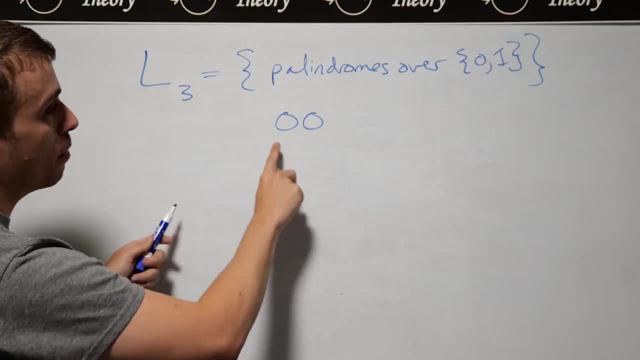 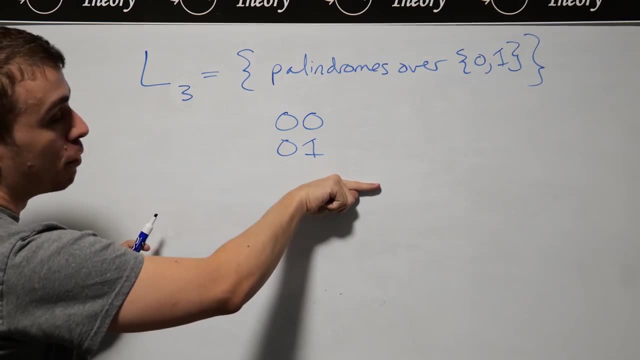 So, as an example, if we have 0, 0, that's a palindrome, because it's the same one way as the other way. If we have the string 0, 1, that's not a palindrome, because in this direction it's 0, 1,. 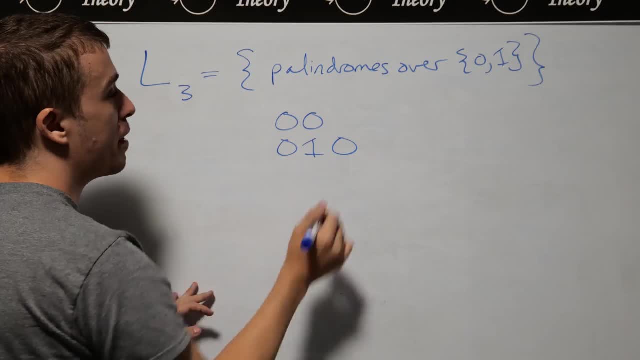 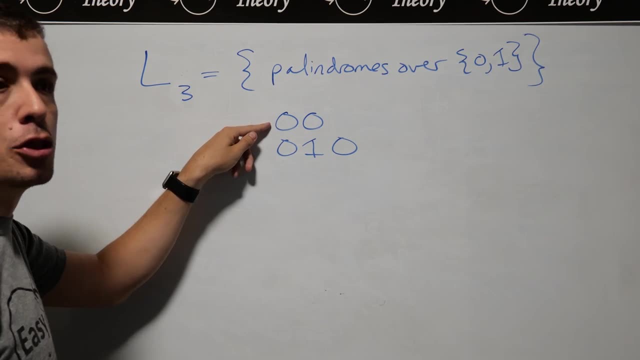 and this direction, it's 1, 0. But if I add a 0 on the end here now, it's exactly the same forwards and backwards, And so note that we could have a string that is of length 2, or even any even number. 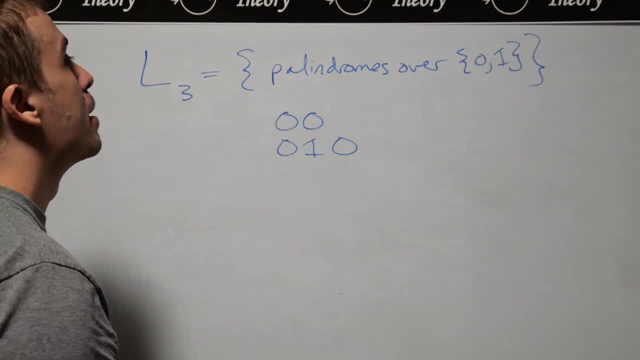 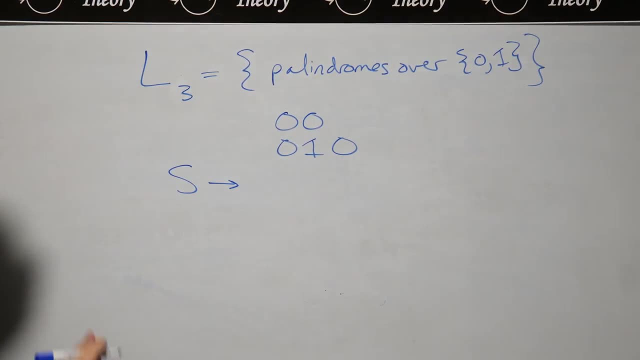 As well as any odd number. And so what we want to do is we want to make a context-free grammar for this. Of course, every context-free grammar has a start variable. So let's make a start variable here And let's think about what a palindrome is. So if we have a palindrome, right, 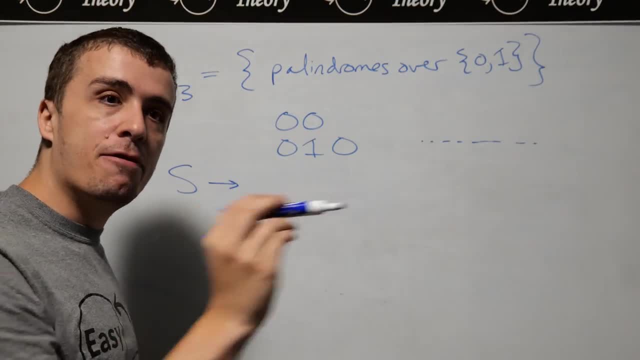 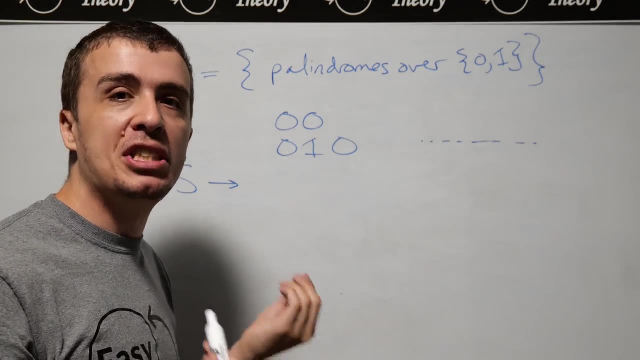 here, then what that means is that it's exactly the same forwards and backwards. Well, if we think about that, if we go this direction and then this direction, we must encounter the same character at the very beginning, In other words, the character at the beginning of the string. 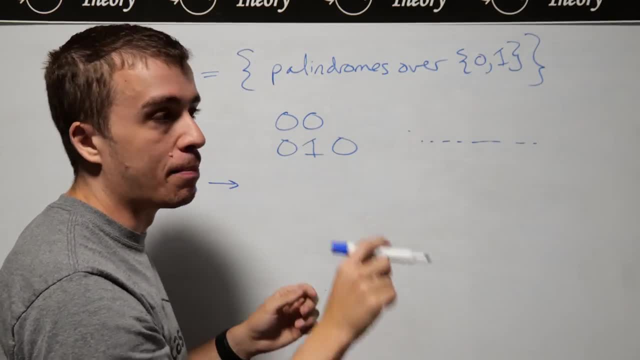 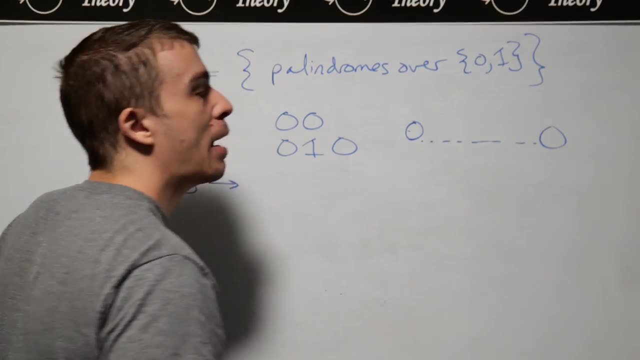 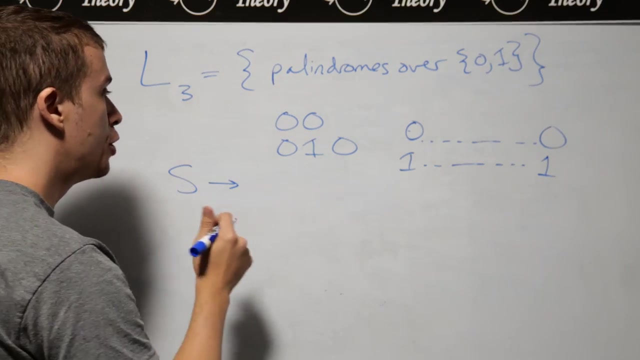 of the whole string is the same as the character at the end of the string, because it's exactly the same forwards and backwards. So if I see a 0,, for example, at the beginning, then I must see a 0 at the end, And if I see a 1 at the beginning, then I must see a 1 at the end also, And so therefore, 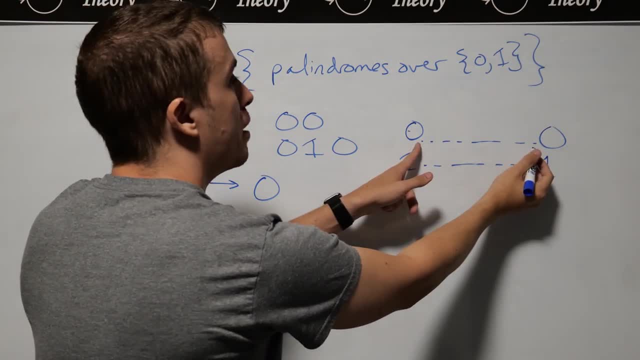 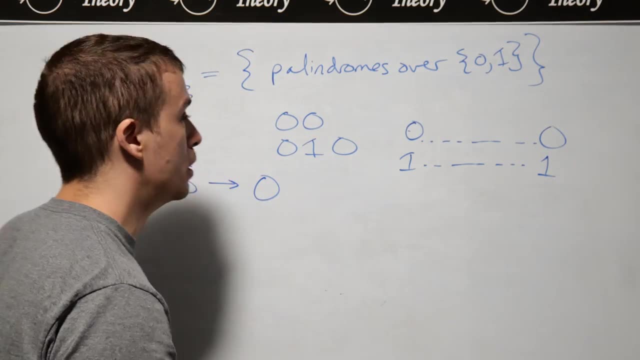 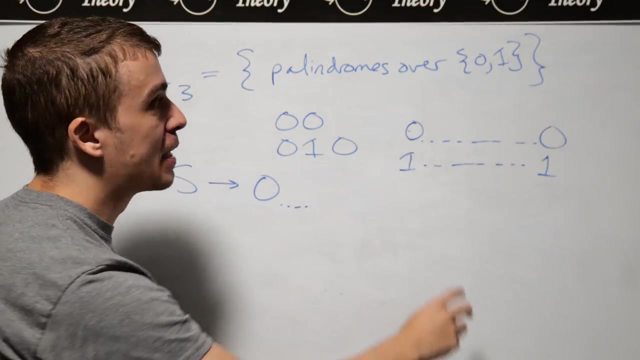 if I see a 0 here, then what must appear in the middle? it must also be a palindrome, because if we take the ends off, it's exactly the same when read forwards as backwards, And so therefore, what goes in here is corresponding to generating any palindrome at all, because there's no. 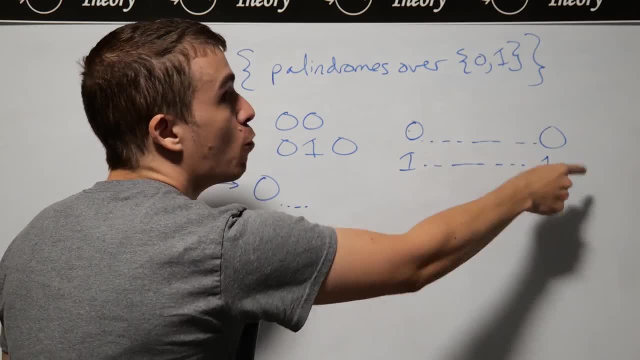 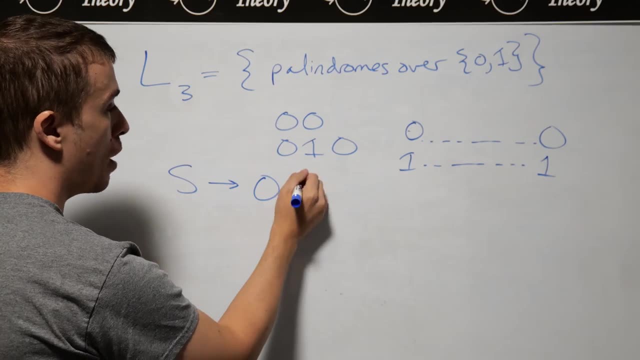 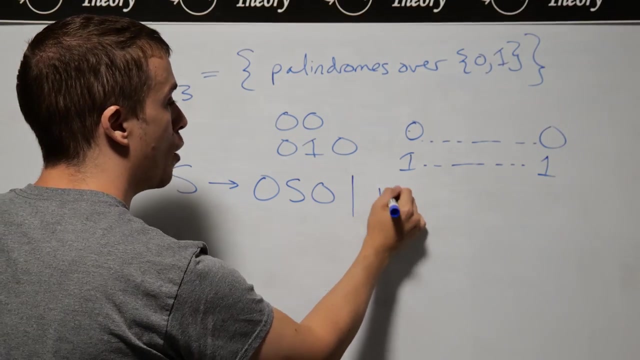 correspondence between what happens in the middle and what happens at the end, And so therefore, if s is going to be representing the set of palindromes, therefore I must put an s here, So 0 followed by some palindrome and then a 0. But also we can have a 1 followed by some palindrome. 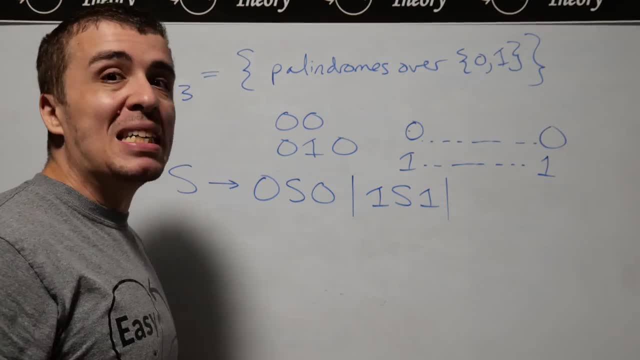 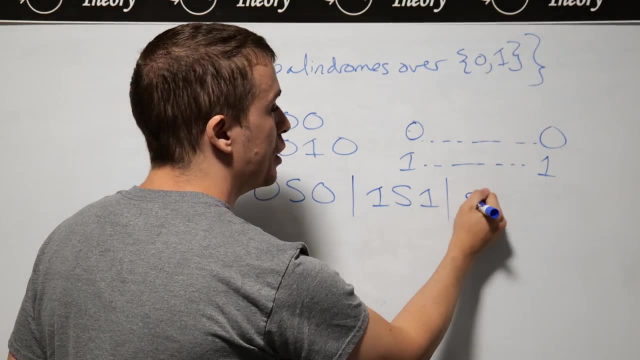 and a 1 for similar reasons. Well then, what's the base case? These are the inductive cases. Well, what are the really smallest palindromes we can have? Well, we can have the empty string. The empty string is exactly the same forwards and backwards. 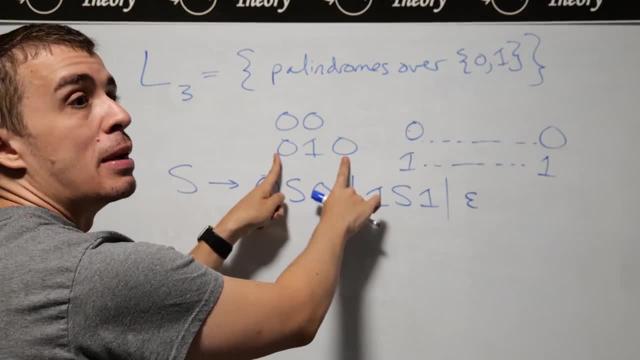 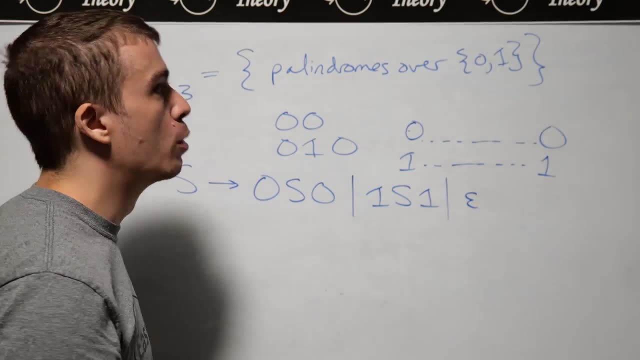 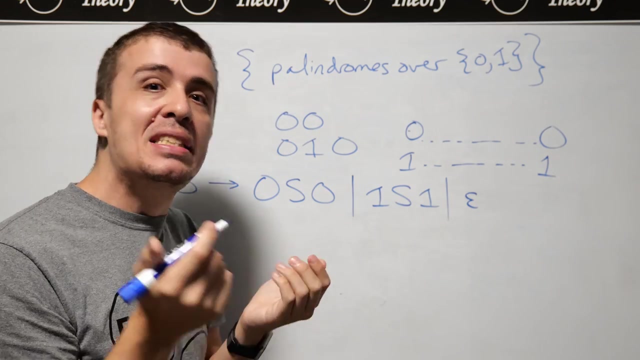 But if we look at what we have here, we'll never be able to generate this string because this has 0 characters and these two rules add an even number, in this case 2 characters. So I'll never get any odd length string. But if we think about a string of length 1, it's exactly the same forwards. 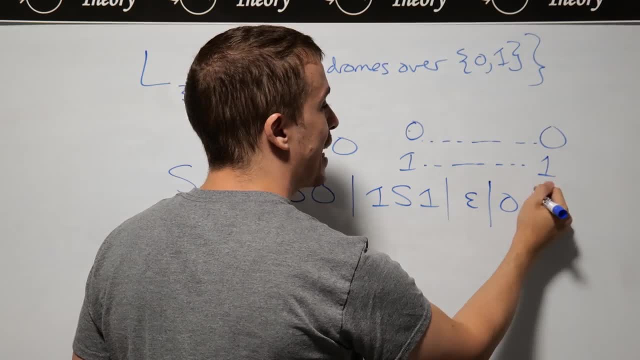 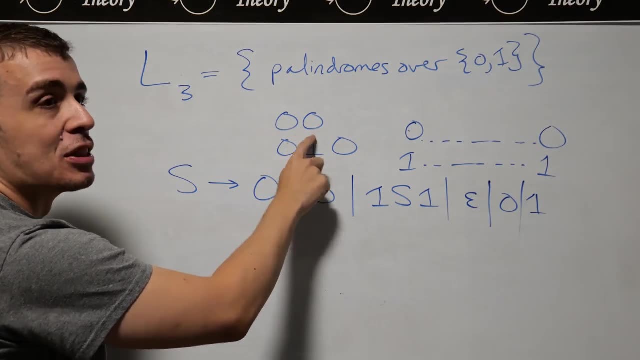 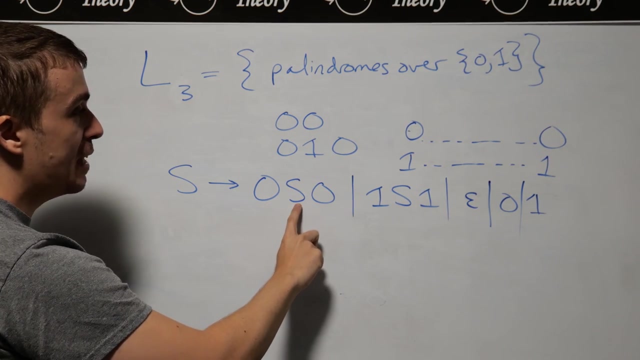 and backwards. So therefore I need to add the base cases of 0 and 1 here. So now let's think: Can we actually generate this string, Because we can obviously generate this string and you should do it for yourself- Can we do this one So that we can apply this rule? then this s can now make the 1 over. 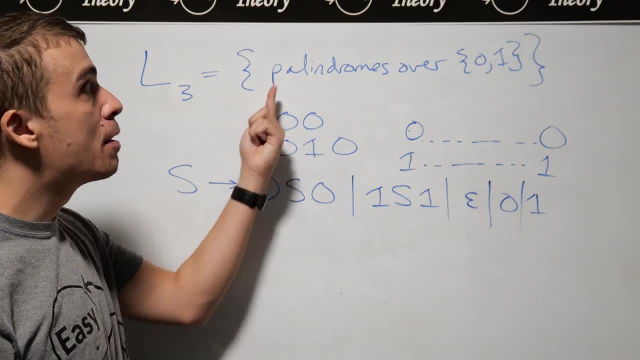 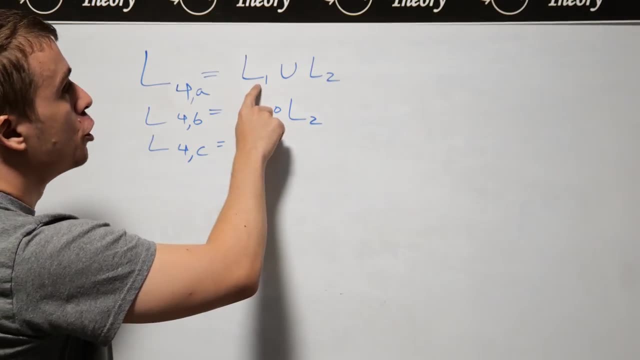 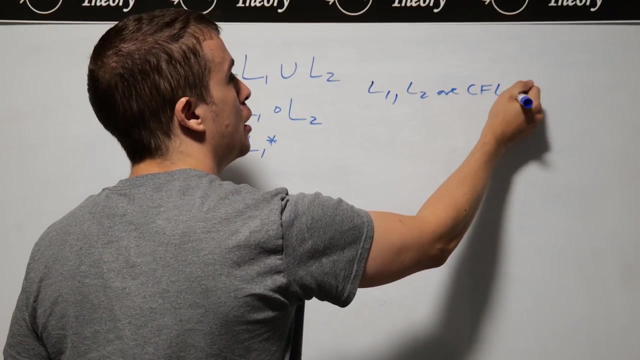 there, And so, therefore, we have made a context for grammar for all palindromes over 0, 1.. So let's make a context for grammar, and actually 3 in this case corresponding to two different languages, l1 and l2, where these two languages are context-free languages. So I have two. 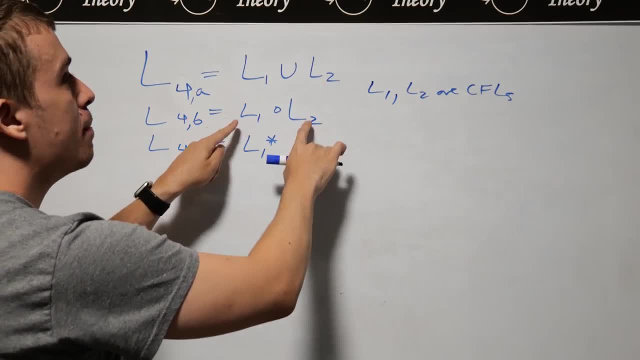 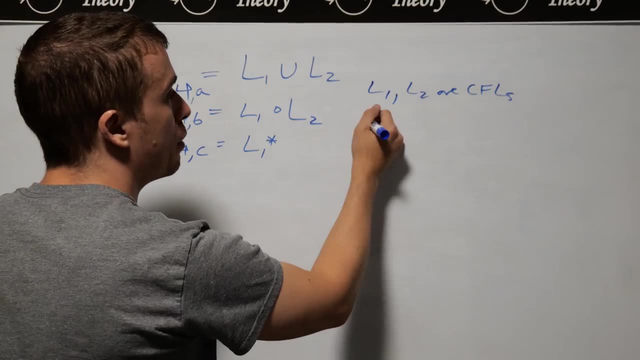 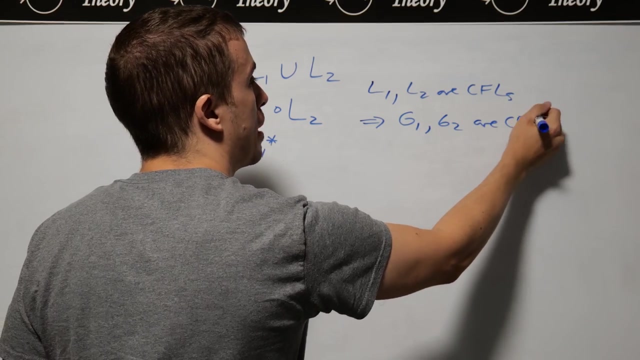 context-free languages and I want to form the union between them as well as the concatenation between them, and then the star of either one, I'll pick l1 here. So if they're context-free languages, then we have two grammars for them. So g1 and g2 are context-free grammars for them. 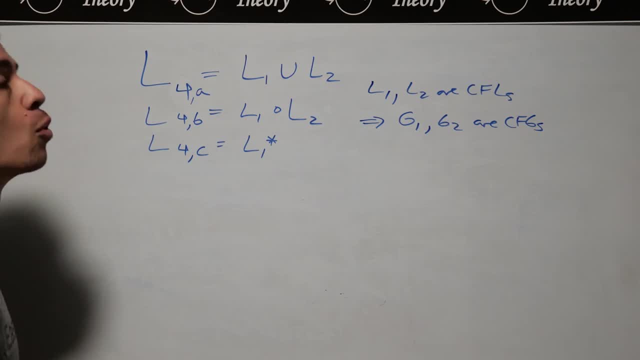 And what we want to do is we want to make a context-free grammar for these 3 certain languages. So let's say that we have g1 and g2, and we want to make a context-free three languages, and it's actually fairly easy to do. So let's talk about the union one first. 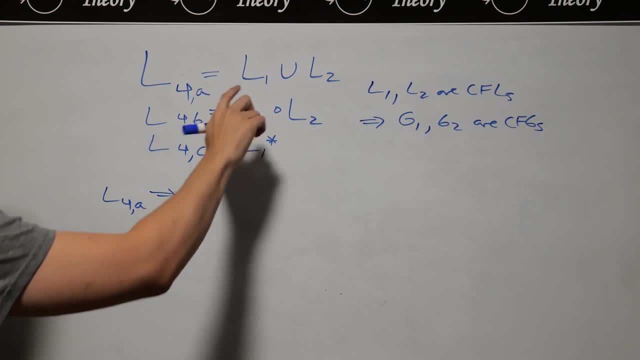 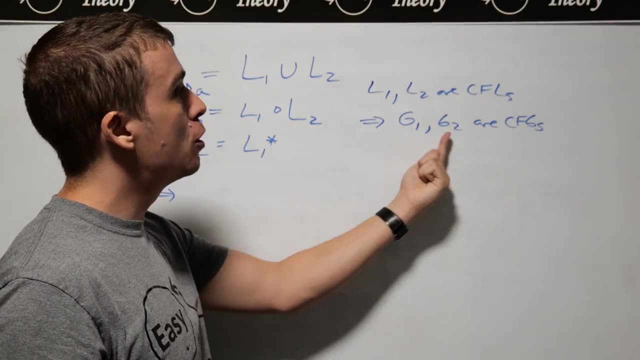 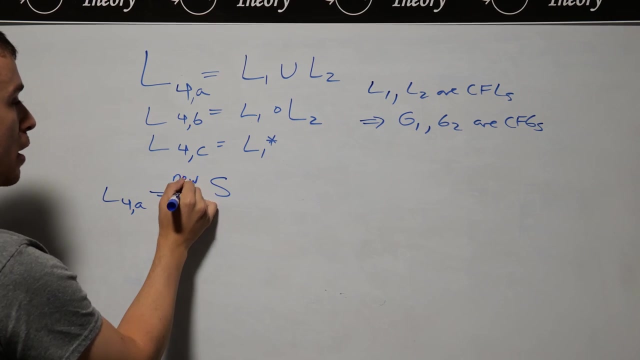 because it actually will generalize. So if we have the union of two context-free languages, then that means that either g1 can make the string that we're after or g2 can make the string that we're after. What we can do is we can make a new start variable. So this is a new start variable. 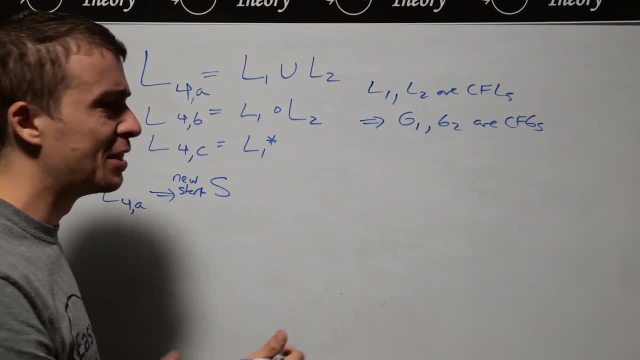 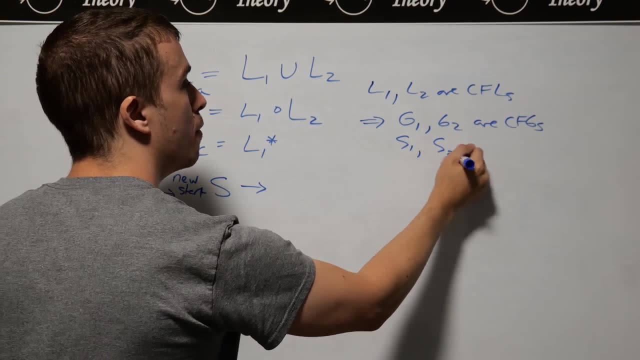 I'm going to call it s here and I'm going to use s in all three cases. So then I'm going to add a rule here that says I'm going to go to the start variable of these two grammars. So let's call them. 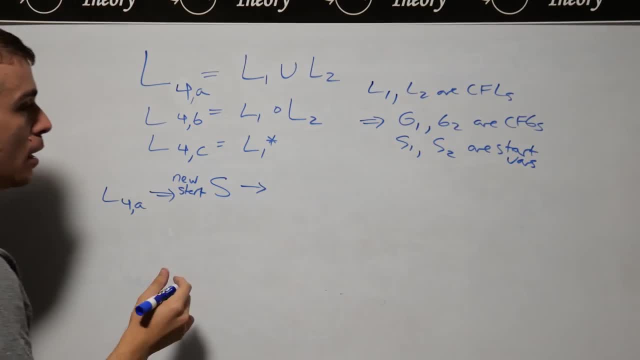 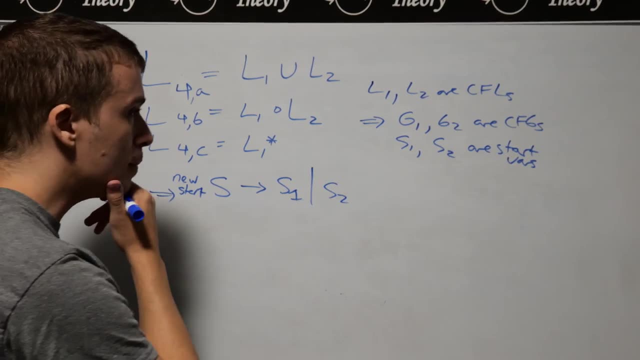 s1 and s2 of these two grammars, Then I can either have s1 make the string that I'm after, or s2 can make the string that I'm after. There's one small technical problem, though, is we got to be sure that the context-free language is going to make the string that we're after. So if we have a 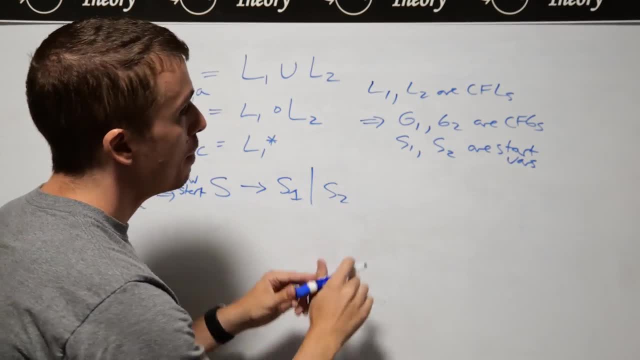 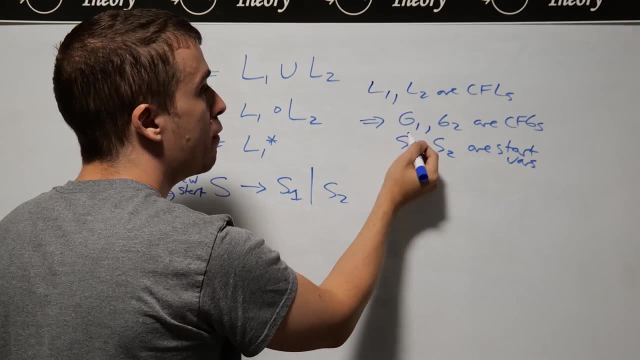 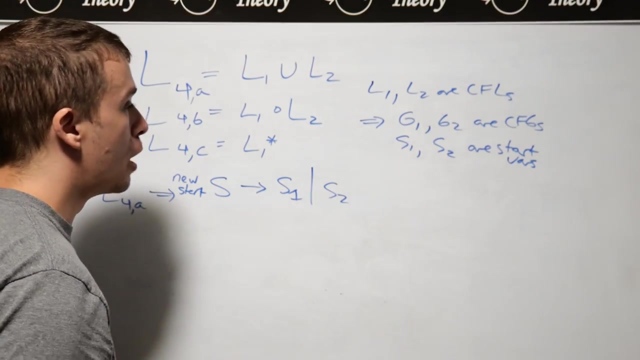 we're dealing with don't have overlapping variables, because if g1 has a variable called a and g2 also has a variable called a, then any rule that g1 involves with a could, in principle, if we just combine the two grammars together, could switch over and that can cause havoc, Whereas 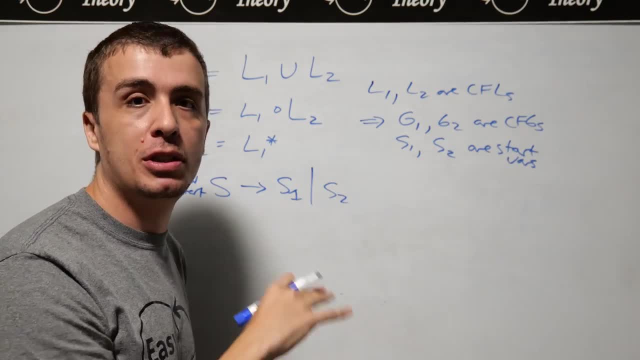 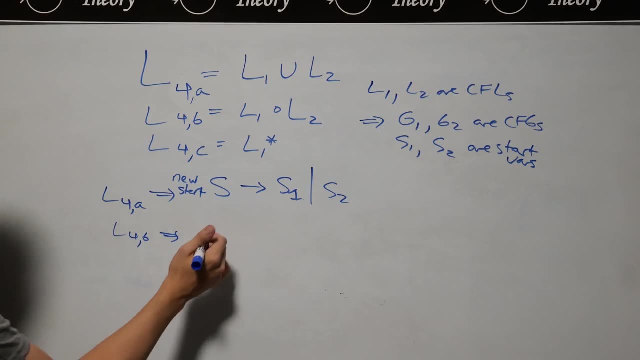 if we rename all of the variables in the grammars, then we have no problem whatsoever. Okay, so now let's do l4b and we can do something very similar. What we can do is, again, a new start variable is still going to be s here, whereas now I'm going to. 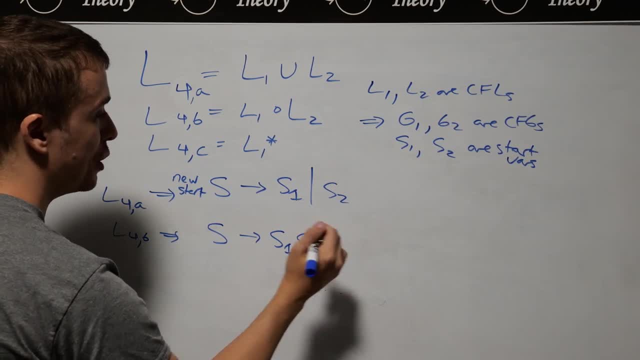 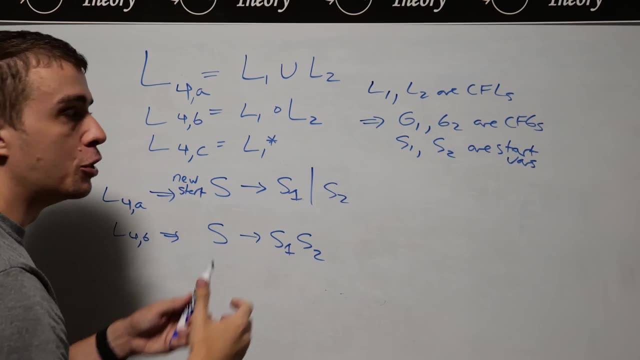 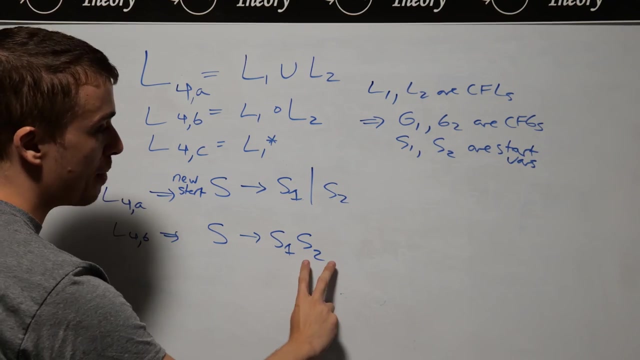 have not s1 or s2. I'm going to put s1- s2 together, because concatenation of two languages says pick a string out of here, string out of here and then combine the two together, Whereas here what we're doing is making some string with s1 and we can't quit early because s2 is a variable and we need 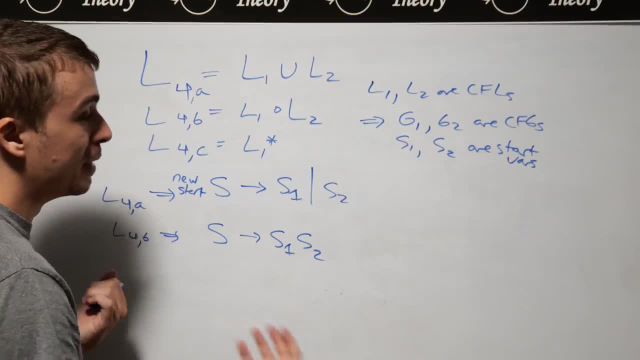 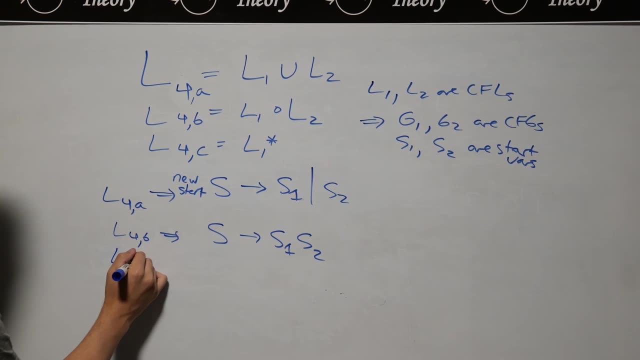 to make a string of terminals. So s2 is going to make some string potentially, So we're going to make a string of terminals, essentially, and then that corresponds to generating a string in the original language. So now let's make one for c and that's l1 star. Well, we got to think: well, what is? 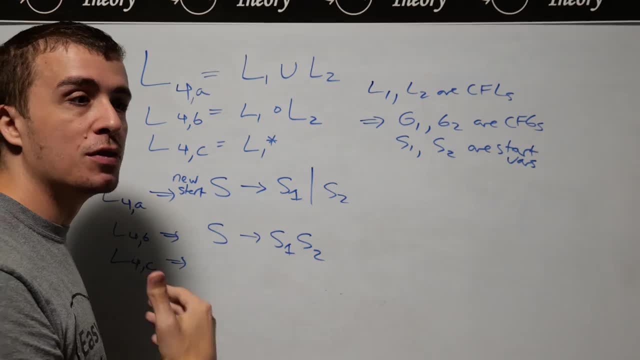 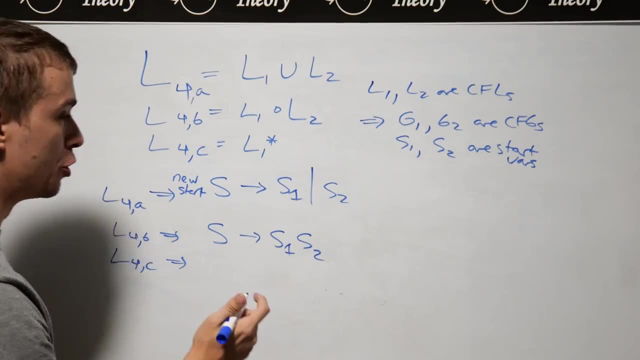 the base case and what's the inductive case, because star involves infinitely many different languages. in some sense, One thing that you should be aware of is that in the star of any language is the empty string. So if we have an s here, it doesn't matter whether l1 can make the empty string. 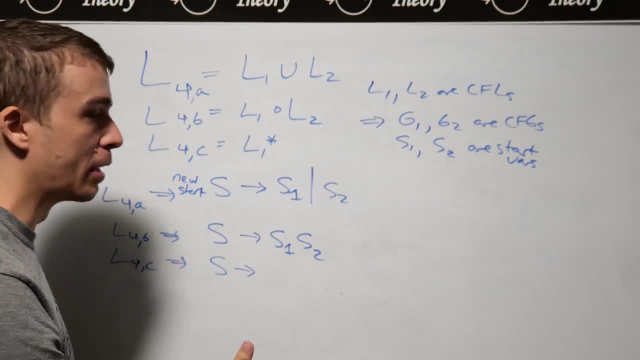 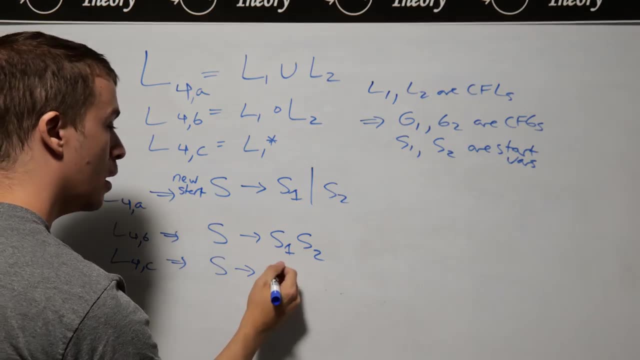 So if we have the empty string itself, l1 star always has the empty string in it. So then this grammar must definitely generate the empty string, even if l1 did or didn't, it doesn't matter. So here I'm going to force that it can make the empty string even if it didn't before. But if we 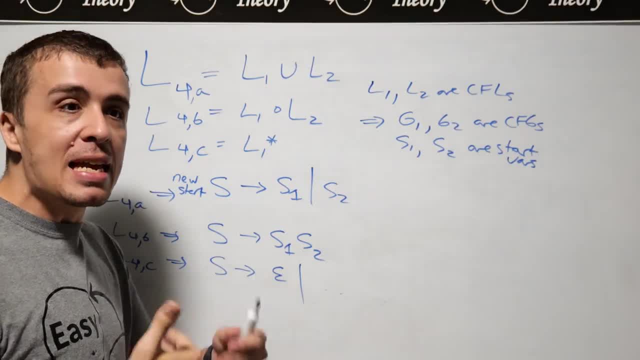 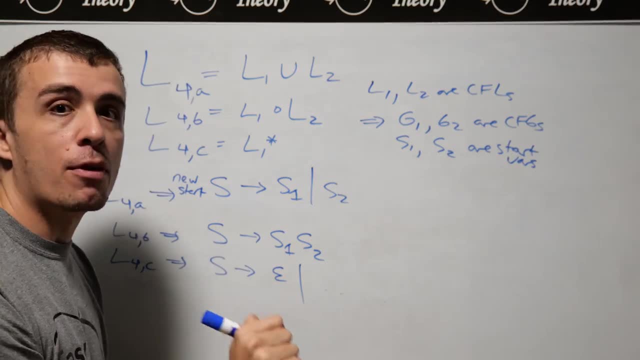 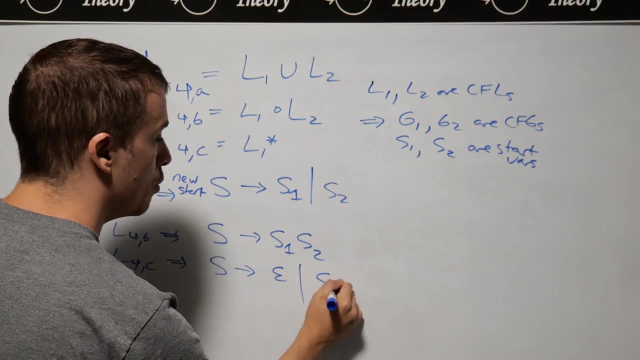 don't do that. well, the star of a language is defined to be any number of concatenations that you wish, And so we can use this idea where we can go down into the grammar for l1,, make a string and then decide: maybe we want to go again if we want to, And so all we need to do is to go into. 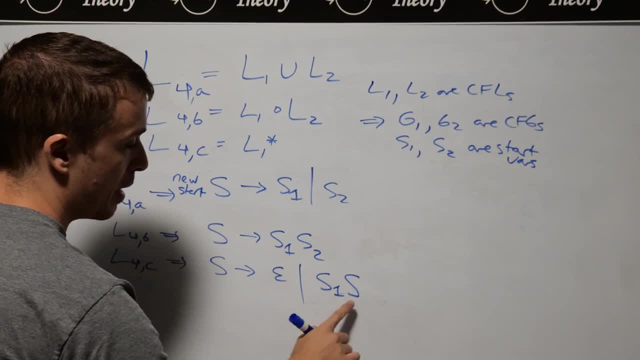 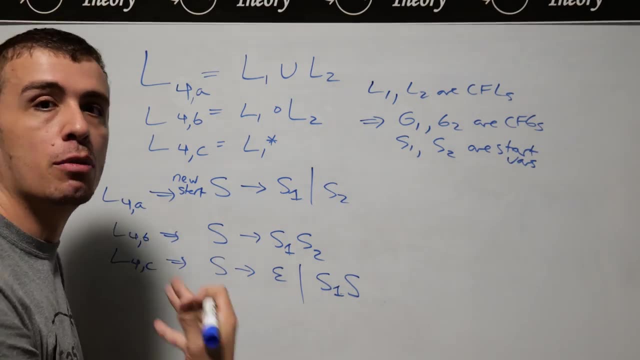 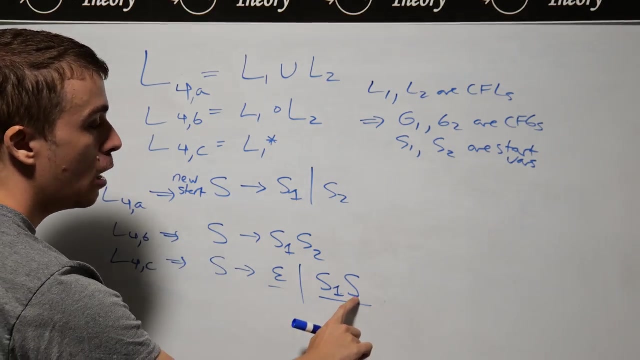 the start variable of s1, followed by going recursively to the start variable here to allow us to go in again as many times as we need to And whenever we're done, we can just make that 1s go away, because whenever we're making this right here, we're only having 1s being generated, which is 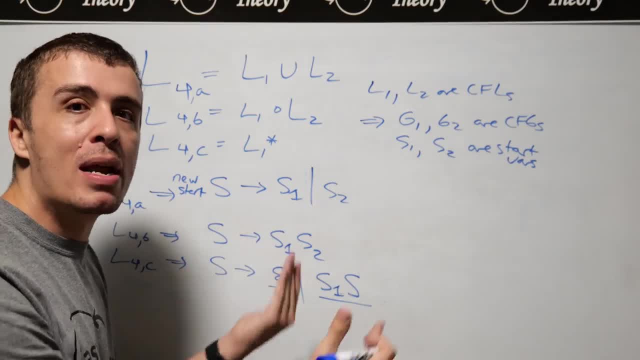 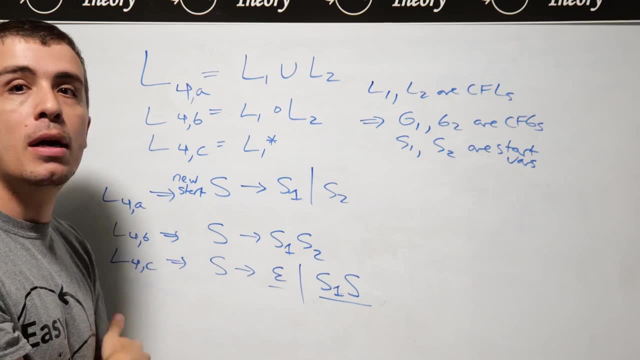 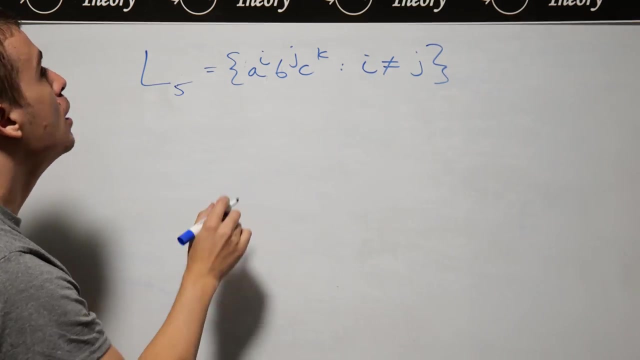 later going to be replaced, So we're going to have, at most, 1s occurring anywhere, which is exactly what we want. So, therefore, we have made a context-free grammar for the union, concatenation and star of two context-free languages. Okay, so let's make a context-free grammar for this language, which is the set of all strings. 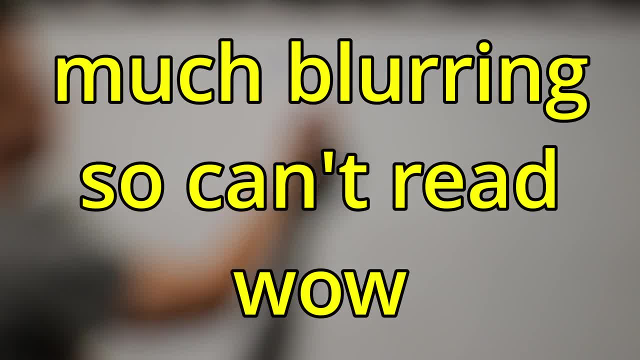 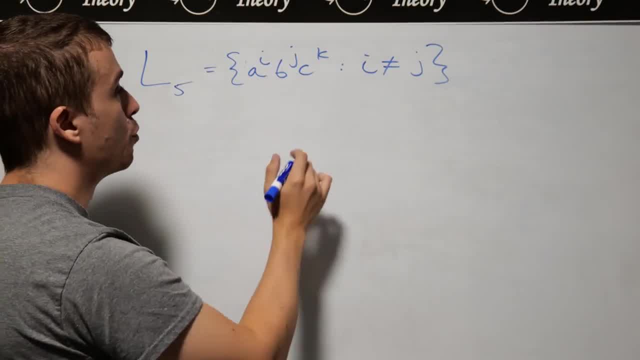 of the form, some number of a's, some number of b's, some number of c's, where the number of a's, which is what i is- is not equal to the number of b's, which is j. And what we want to do is: 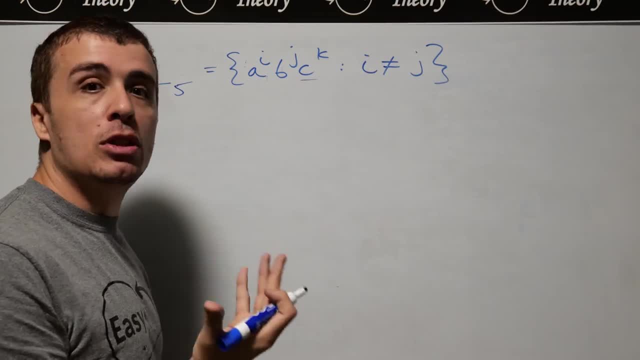 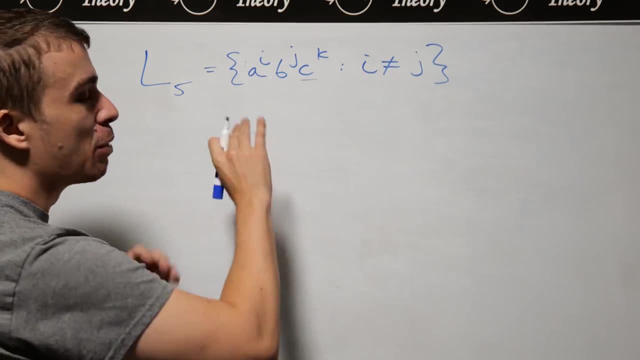 to make a context-free grammar for this. Notice that the number of c's here, which is k, has no relation to the number of a's or b's, which are i and j here. So what we can do is we can forget about the c's and we just focus on the a and b part, and then d. we can just focus on the a and b. 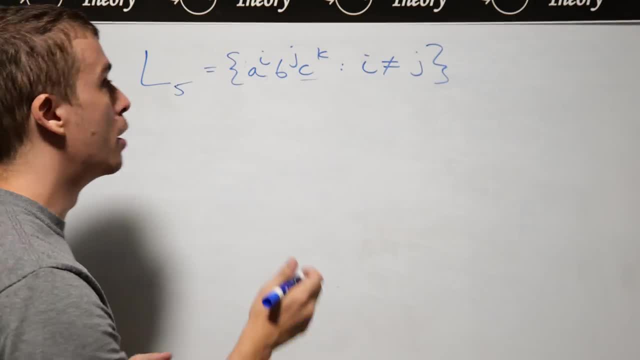 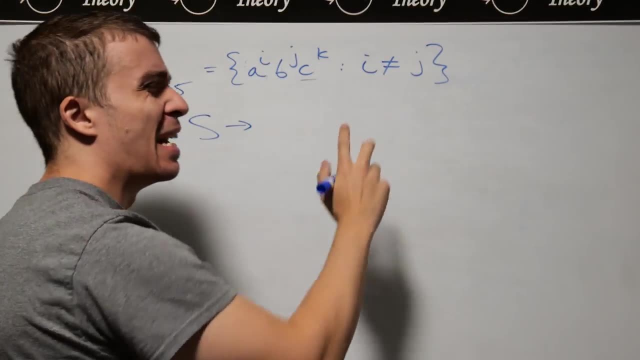 part and then deal with the c's later. So every context-free grammar has a start variable. so let's make a start variable here and i'm going to label it like this. So let's think about how we're going to structure this. How do we actually tell whether or not? 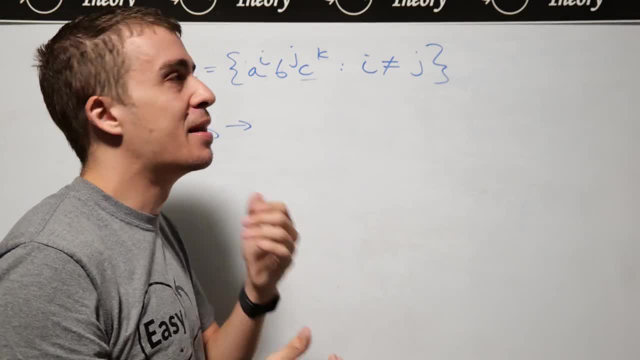 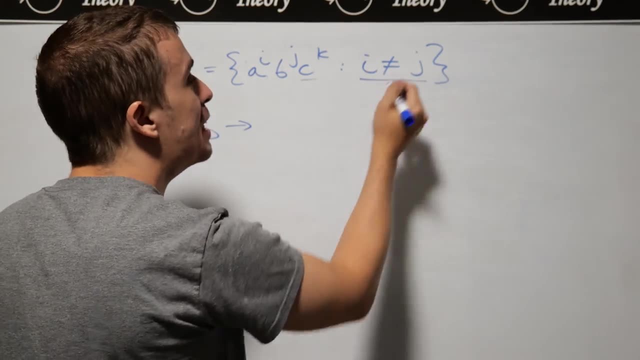 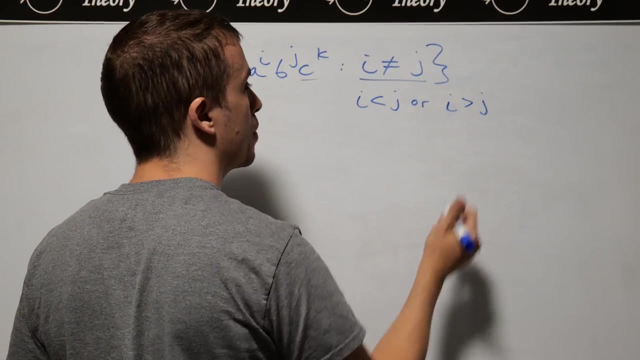 the counts of two variables are the same or not. That seems a little weird. All that we need to do is to think about this in a slightly different way. Another way of rephrasing this same condition is to say: i is less than j or i is bigger than j. It must be one of those two, because they can't be. 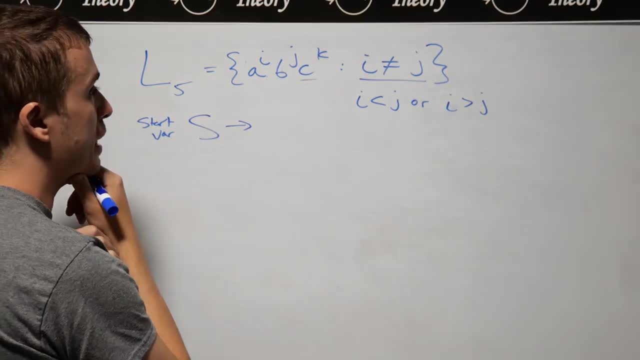 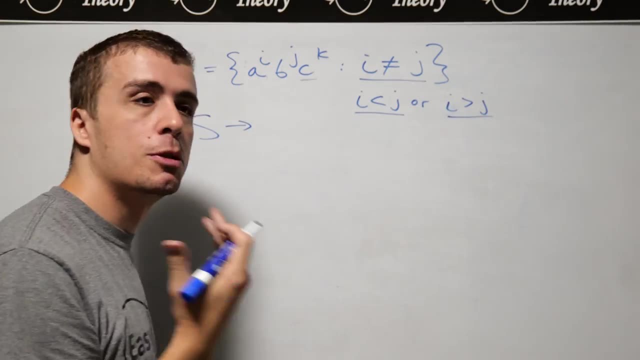 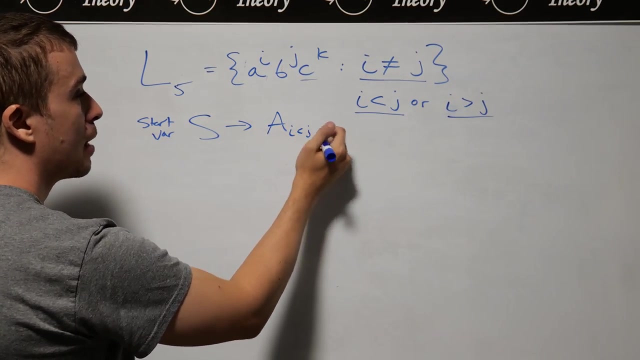 the same. So how are we going to relate these two together? Well, we're going to have a variable that corresponds to the i less than j case and another variable that corresponds to the i bigger than j case. So I'm going to have two variables called a i less than j. You don't have to have 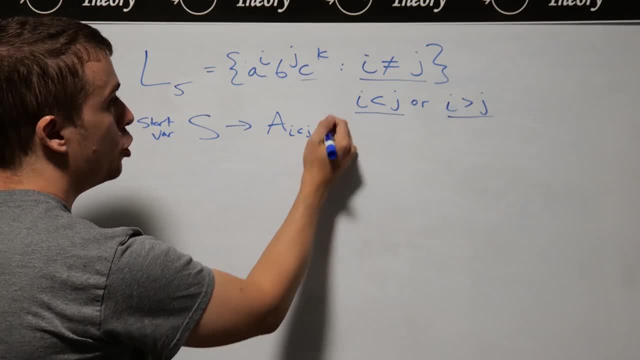 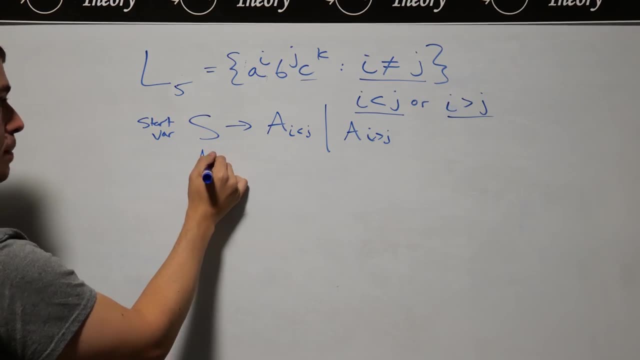 the subscript here. It's just to help you: a i less than j or a i bigger than j. So let's deal with the i less than j case. So i less than j. Well, that means that the number of a's is less. 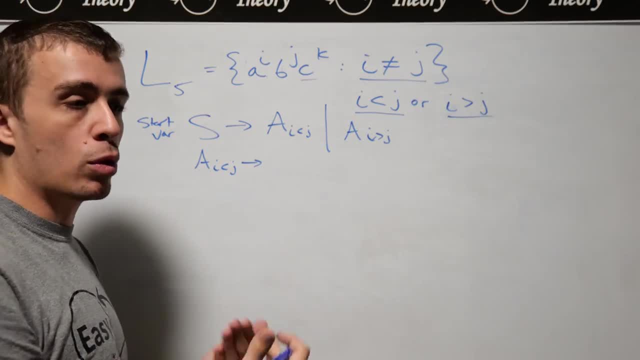 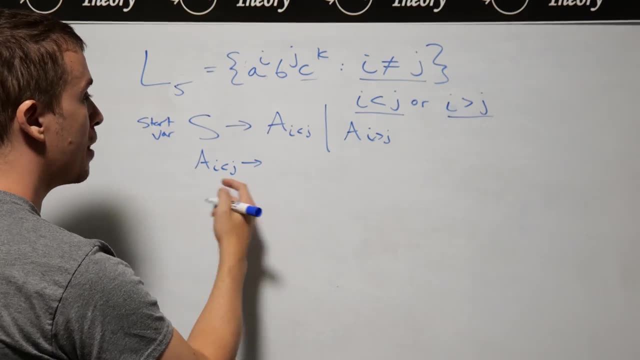 than the number of b's, But the number of b's could be only one more than the number of a's, or way more than that. It could be anything in principle. So what I'm going to do is I'm going to allow ourselves to make a's and b's. 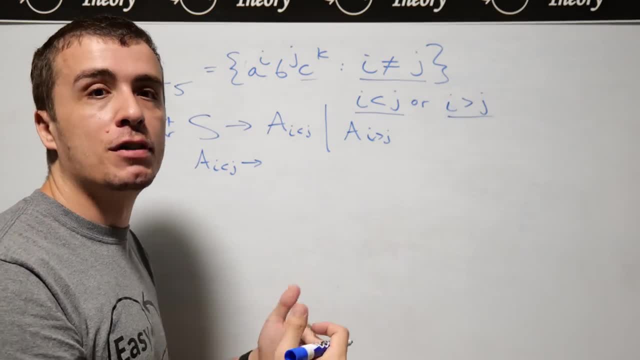 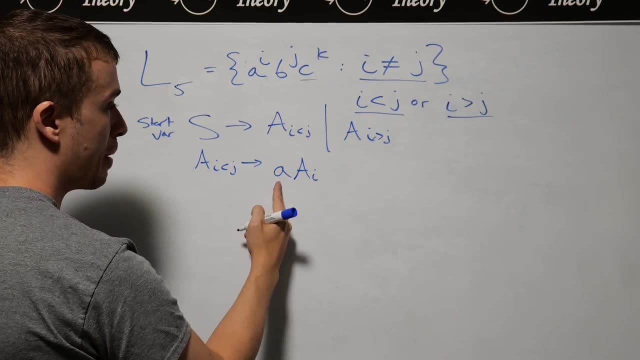 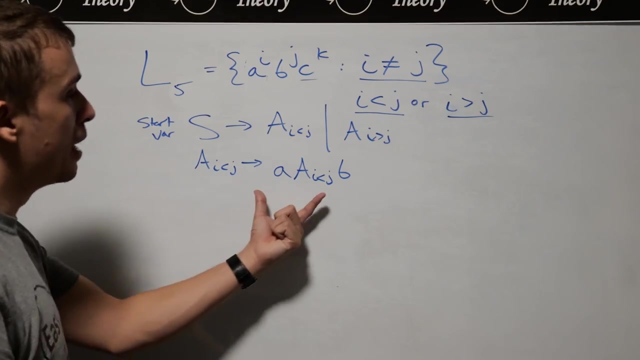 an equal number and then later allow ourselves to make as many more b's as we need to. So I'm going to say I'm going to have a rule like this. So I'm going to generate one a here, recursively, go into this same variable with a- b. So that means that I'm going to have a rule like this, So I'm going to 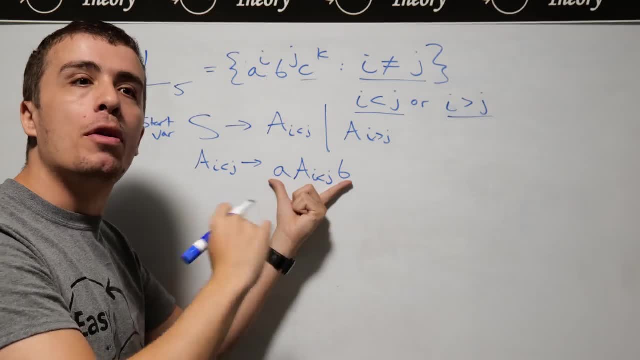 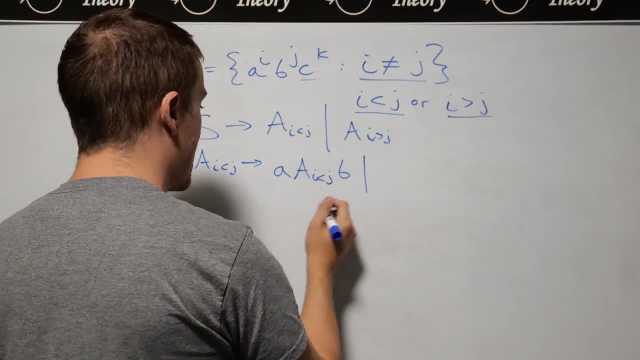 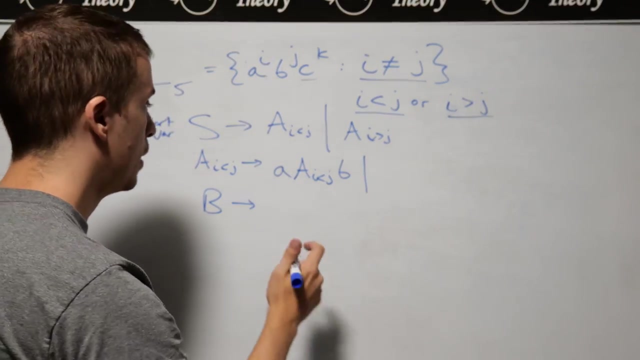 at this point be generating them in equal numbers, So one a for every b, but of course we got to make at least one more b. So then I'm going to have a variable right here which is called making b's, or I'm just going to call it b here, And its sole purpose is to make more b's. That's it. So I'm. 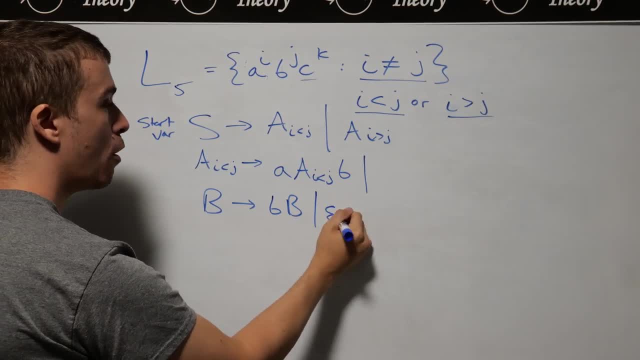 going to have more b's right here. So this variable b is just going to spout off as many b's as it wants- at least zero, And it's important that it's at least zero. You can work it to where b makes. 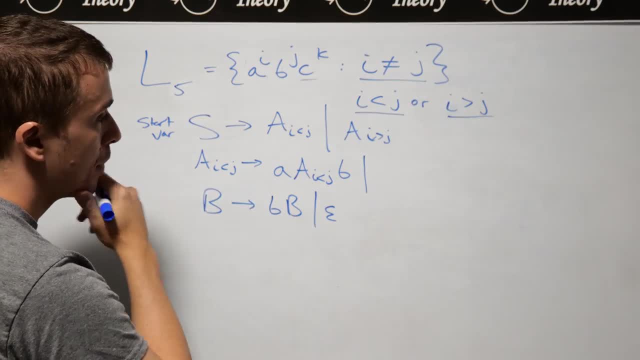 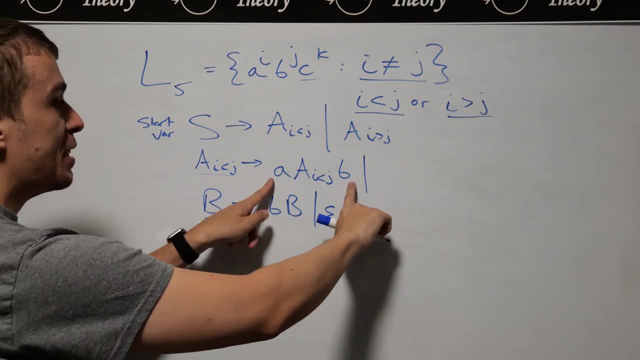 at least one more, But I'm going to do it this way. Well, how are we going to relate the i less than j guy to the b guy? What I'm going to do is notice that we have the same number right here, and this guy only guarantees to get at least. 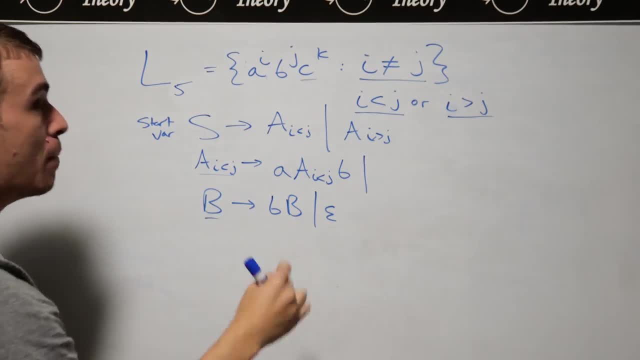 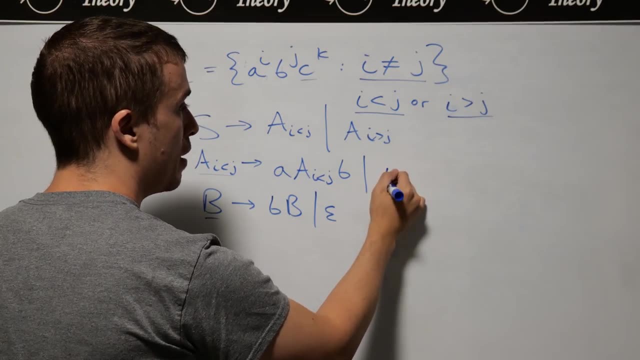 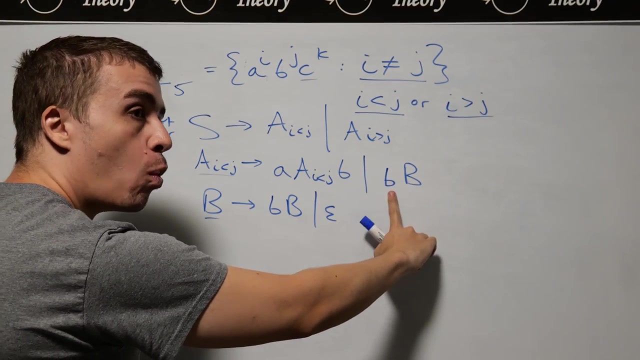 zero more b's, Whereas a, i less than j, must generate at least one more b, And so, therefore, to get down to here, I'm going to have this be my rule. So, in order to make a string at all, I must have at least one b right here which does not correspond to an a, And so therefore, 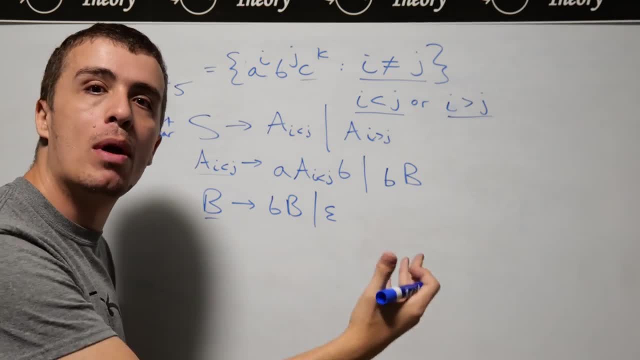 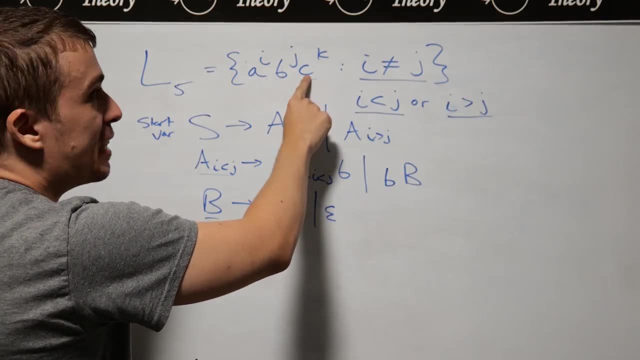 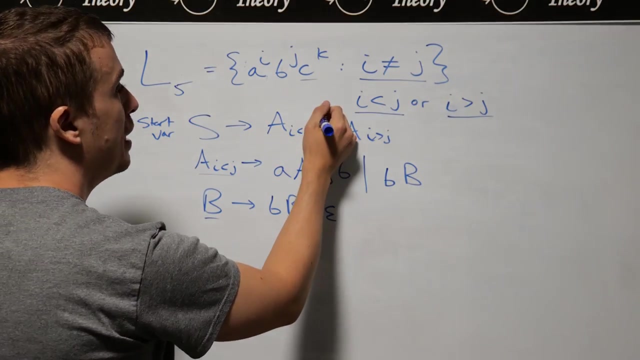 whenever this makes a string, I must have at least one more b than a, which is exactly what we want. Well then, now the only thing that we have to deal with is dealing with the c's at the end, But again, they don't have any relation to the i and j numbers, So one easy way of doing this.